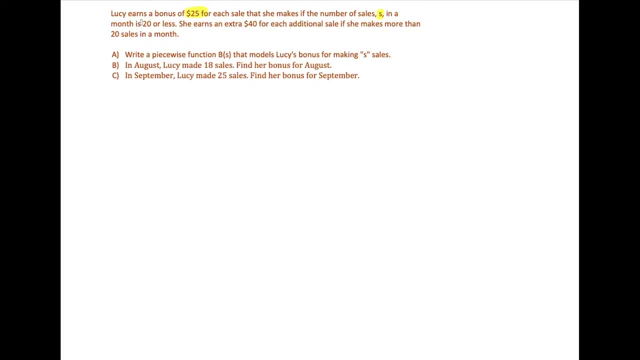 but she gets a $25 bonus for each sale if she makes 20 sales or less, And the next part here now: she gets a $40 bonus if she makes more than 20 sales a month, And the first thing we have to do is write a piecewise function that models Lucy's bonus for making S sales. So a few things. 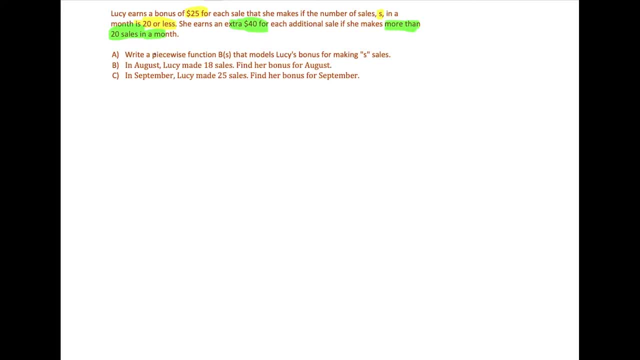 we have to be mindful of here. Well, for one, that when Lucy makes less than or equal to 20 sales a month, she gets a $25 bonus. So that tells us that B the amount of bonus that she gets is equal to 25 times S. So really all. 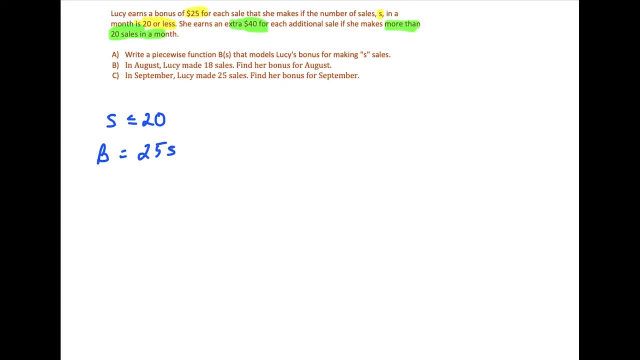 we're doing is if she makes one sale, she gets $25.. If she makes two sales, she would have 25 times S equals two, which would be a $50 bonus. So this part here isn't too bad, but where things 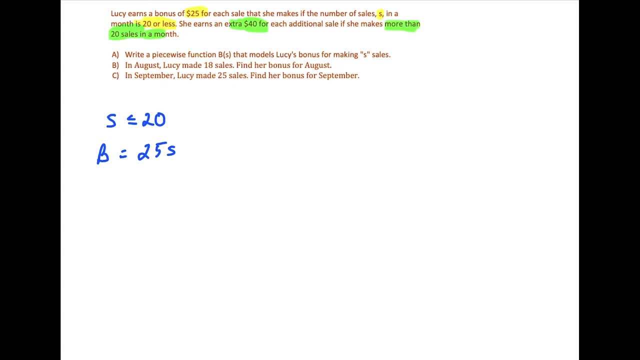 get a little bit tricky is when we consider the next part. What happens when she makes more than 20 sales in a month. So for the S greater than 20 scenario, well, there's a few things that we have to consider. That the 21st sale she makes $40 per. 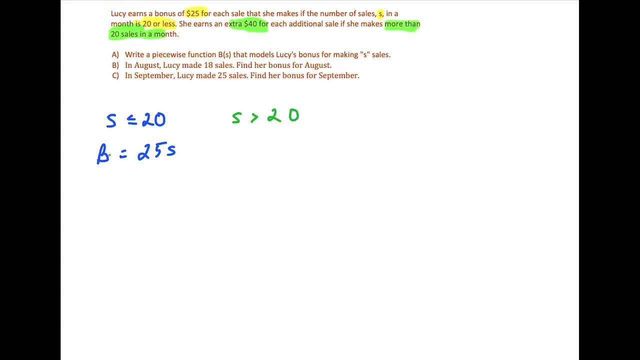 sale. for every sale more than 20, but we still have to account for the first 20 sales. So for the first 20 sales, Lucy makes B equals 25 times 20.. So we're essentially just using our first equation here And that 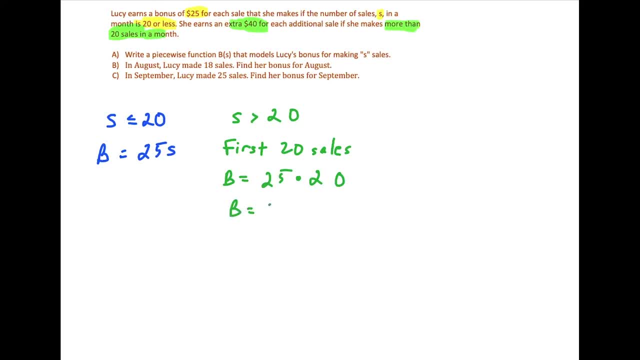 tells us, when we multiply this out, that Lucy makes $500 in bonuses if she sells 20 items. So that's something that we have to be very mindful of here, because now for the 21st sale, she's going to make $40 per sale. 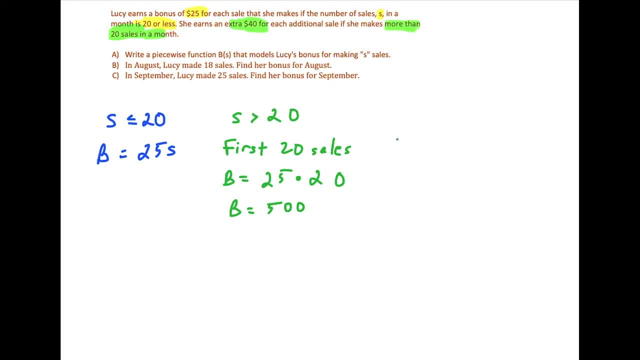 So this is very important. So, when we have to set up the second equation- and remember this is for when S is bigger than 20.. Well, the starting amount she already made $500. So remember, all we did was multiply the 20 sales by $25, which represents the bonus to. 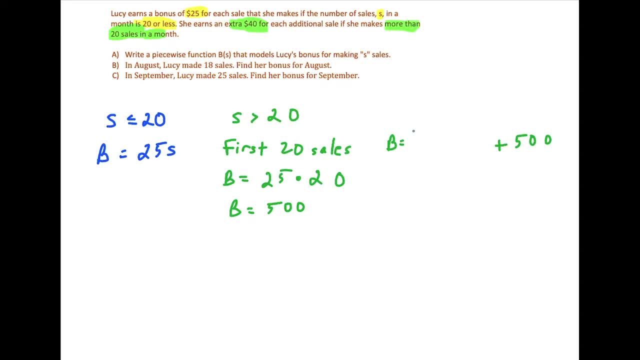 tell us that she has a $500 bonus, But now, instead of multiplying S by 25, now we're to be multiplying by 40, because the bonus increases. that's the incentive. the more items you sell as a salesman, then sure they'll reward you more. so now she gets a 40 bonus. but this is. 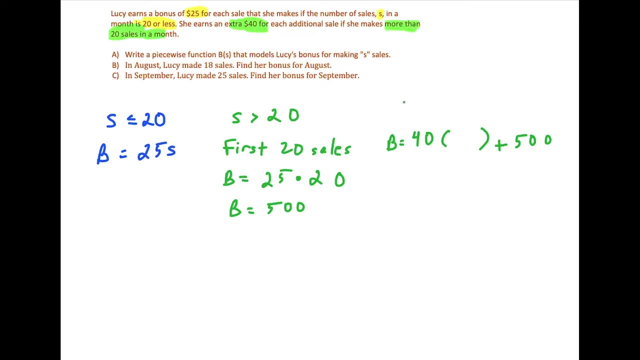 where we have to be careful for this section here. what we have to think about- so this wouldn't necessarily be part of our work like this is what's kind of going on in your head here, but i want you to think about this. when she sells 21 items, this is one sale above or over. 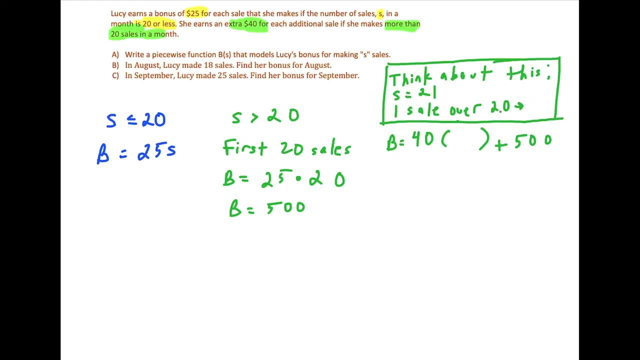 20, which, if we just do that quick math in our head, well, if she makes 40 dollars per sale for every sale over 20, she makes 500 for selling 20 things. so 500 plus 40 that's going to earn her 540. 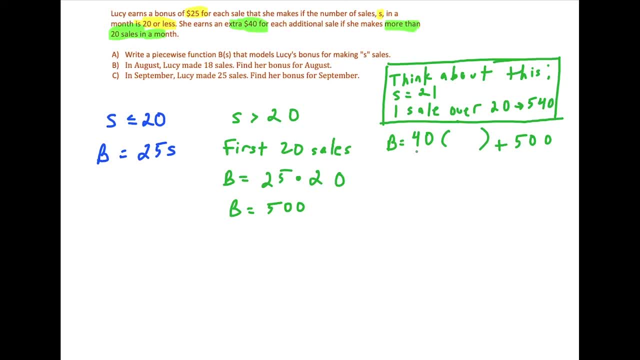 so this forward thinking and word problem does help you set up the correct equations. so if we think here, what this tells us is that when we plug in s equals 21, we should wind up with 540. So the problem with just writing s here is that s equals 21,. 21 times 40 plus 500 is way, way, way over 540. so we have to be very careful. 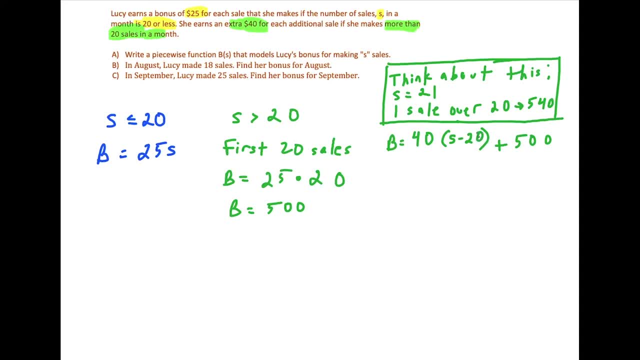 so we're going to throw in an s minus 20 here, because remember what i just said to think about: when we plug in a 7 billion dollar sum- and we do that- we're going to find out that 7 billion is s equals 21,. we should get 540.. And when we plug in 21,, 21 minus 20 is 1.. 1 times 40 is 40,. 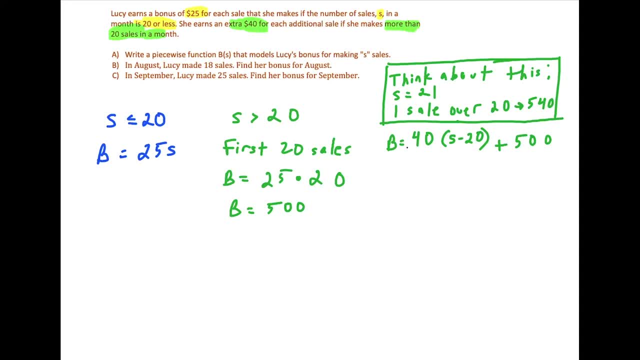 plus 500 gives us the 540.. Okay, so now we're ready to combine these two equations from these two different domains to write our piecewise function. So we're going to name our piecewise function b of s And we'll draw in our brackets And we're going to write the first domain first. 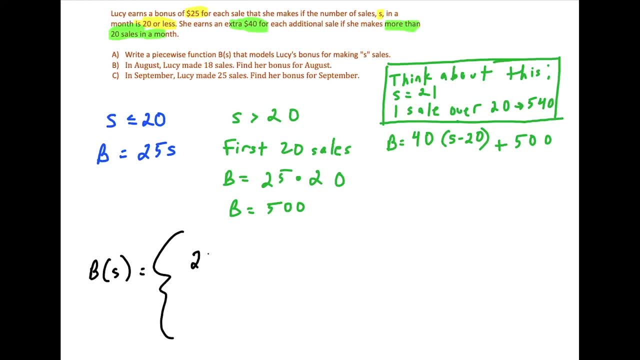 When s is less than or equal to 20,, the equation is 25 times s. And for the next domain, when s is greater than 20, we have 40 times s minus 20, plus 500.. And remember, this is for when Lucy makes more than 20 sales. 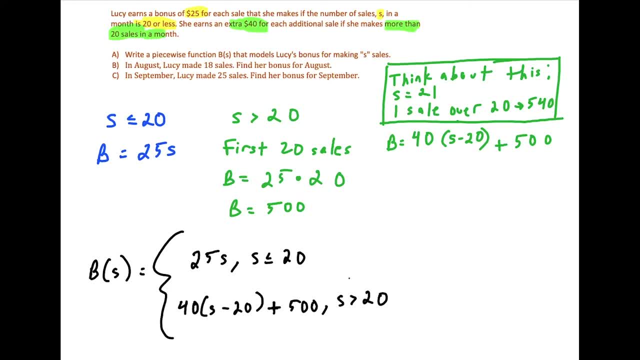 Okay, and once again this function does make sense, because when Lucy's makes more than 20 sales, it accounts for the fact that she already made 20 sales, So she has $500 of profit already locked in. So now this completes part A for us, And now part B and C. 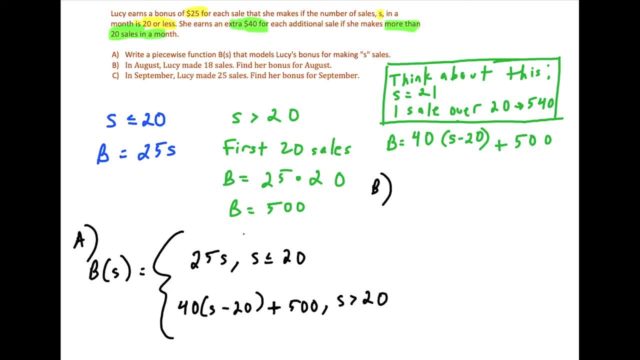 are fairly simple, because now all we have to do is plug into this formula we just created. So in August, Lucy made 18 sales. Find the bonus for August. Well, now we just plug in 18 to our function And when we plug in 18,, we get 18.. And when we plug in 18,, we get 18.. And when we plug in 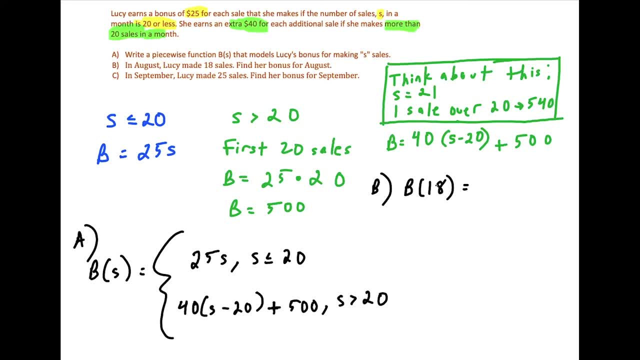 to a piecewise function. the first thing we have to determine is: where does 18 land? Is 18 in the first or second domain? And since 18 is less than or equal to 20, we're going to plug 18 in for this. 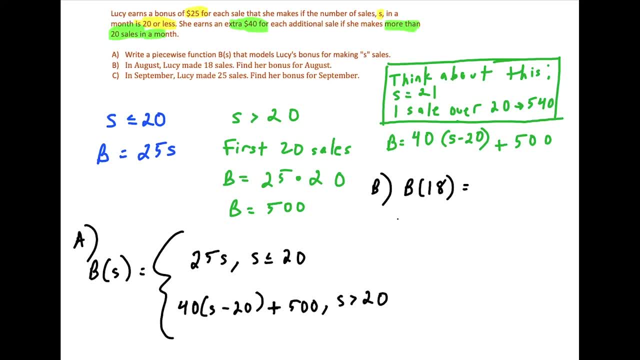 part here 25 times s, we're going to have 25 times 18.. Okay, so to simplify this, we could use a calculator, Or you could just do the multiplication in your head. Either way, But 25 times 18 is 400.. 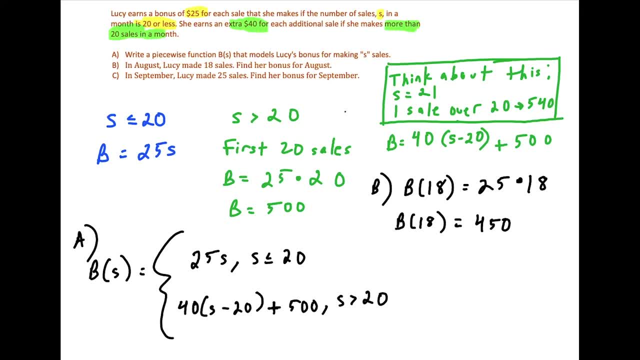 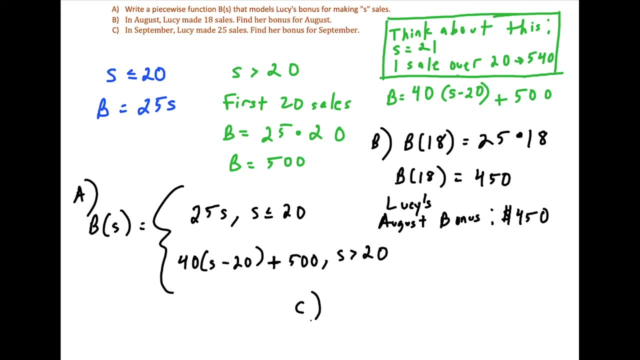 So then we want to find her bonus for the month of August. That tells us here that Lucy's August bonus is $450.. Okay, now the last thing to look at here for part C is we want to calculate Lucy's September bonus, And Lucy made 25 sales in September. So if we evaluate our function B of s, 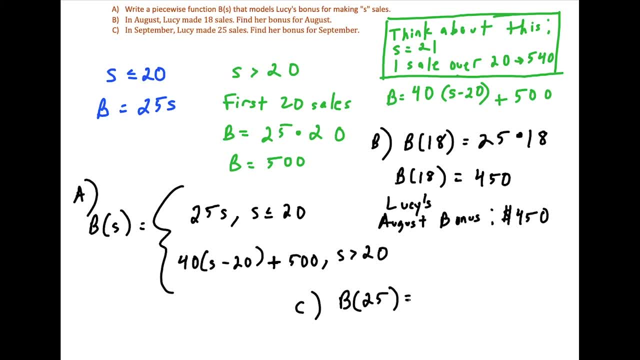 at s equals 25,. well, once again, we just have to say where does 25 fit in the formula, In the domain, And 25 is greater than 20.. So we would plug in s equals 25 to our bottom equation.